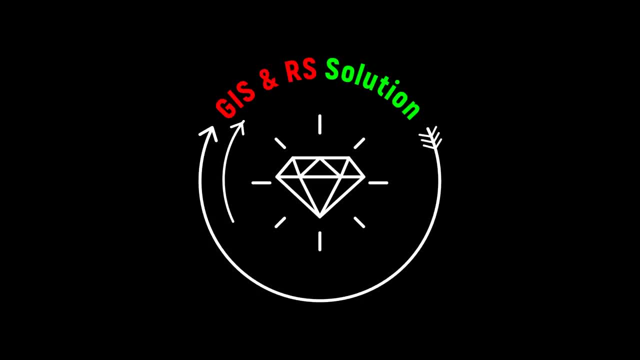 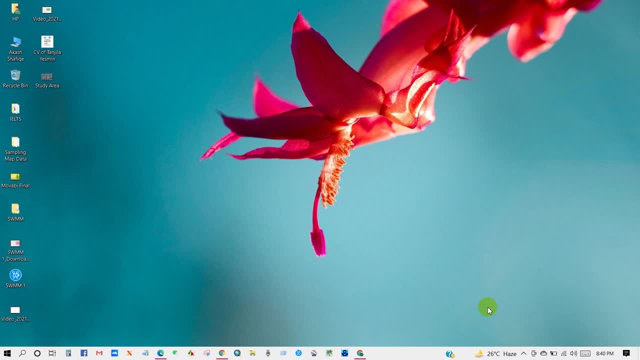 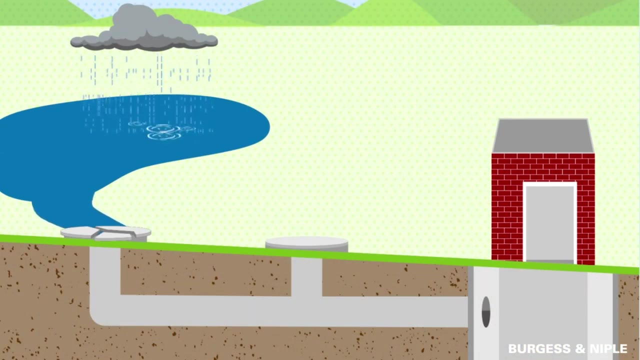 Hello, dear viewers, Hope you all are doing good. Besides GIS and remote sensing, I upload several video tutorials on environmental and disaster modeling data analysis using significant recognized software. Anyway, here I'm back with another new video on stormwater management model. In the previous video I have showed you how to download and install SWMM 5.1 version and explained the use of it. 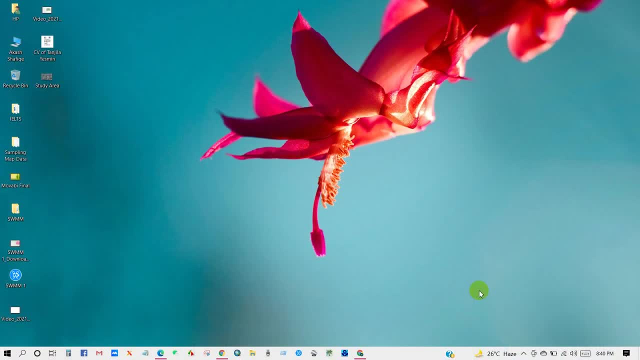 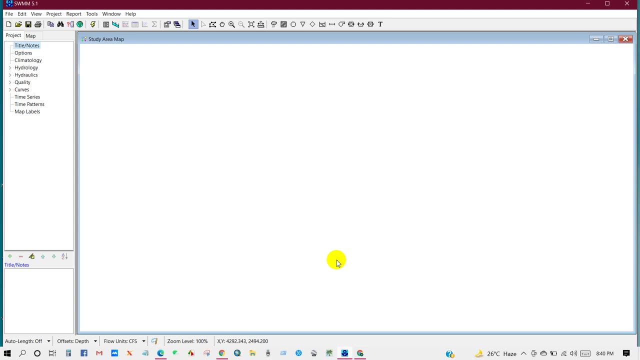 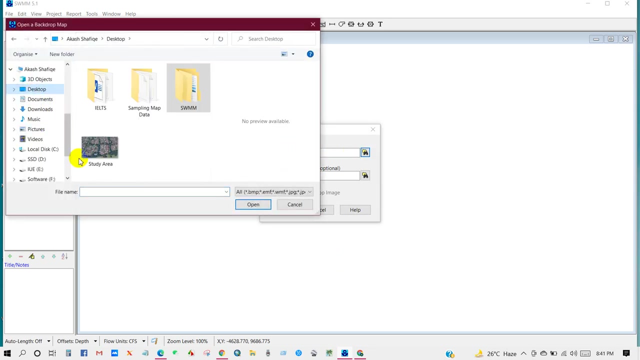 In today's video you will learn a complete project where I will show you a design of urban drainage system. First, open software SWMM, Then I will add raster file of my study area For that go to view. then backdrops load, then backdrop image file. I'm adding raster file of my study area. Then click open and then click OK. 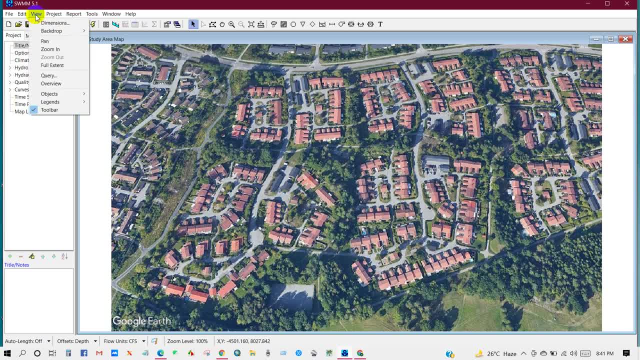 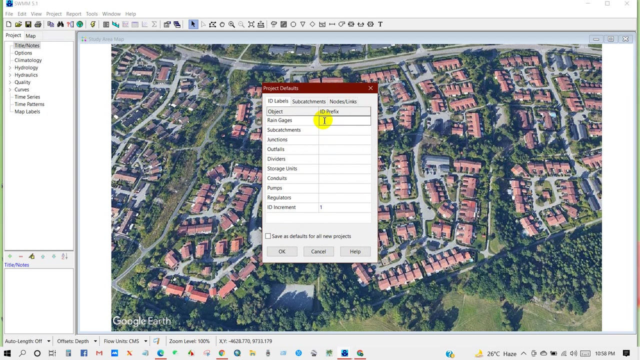 And then go to view dimensions, Check meters as map units, Then flow units. It is in CFS, It is in cubic feet per second. I will change this as CMS: cubic meter per second As flow unit. Then go to project and then defaults. You can see here ID levels, object and ID prefix. I will set for ranges is R, then subcassment AS junctions, J, then outfalls PO. 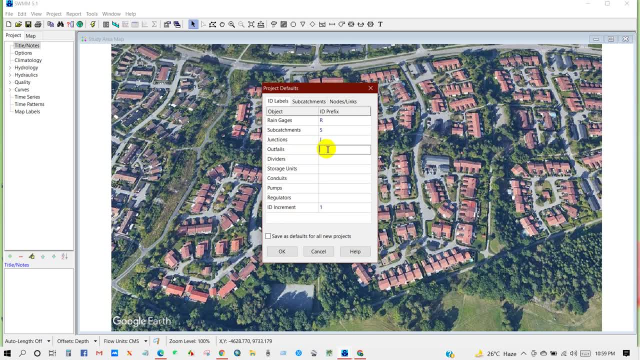 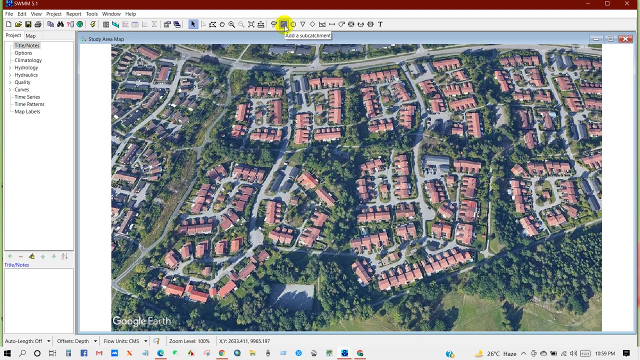 Save as defaults for all new projects. You can check this on conduits C, Then click OK. Now subcassment. So what is subcassment? A subcassment in the network represents the physical area from which a manhole or other inflow node collects water. 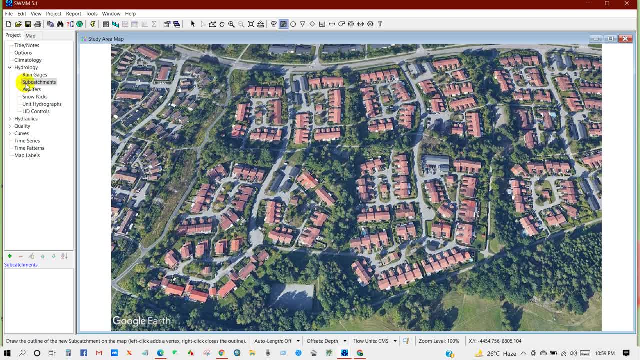 And in other words, you can define subcassments as hydrologic units of land whose topography and drainage system elements direct surface enough to a single discharge point. The user- I mean we- are responsible for dividing The study area into an appropriate number of subcassments and for identifying the outlet point of each subcassments. in this design- I mean in this exercise- I will draw three subcassments for my study area. 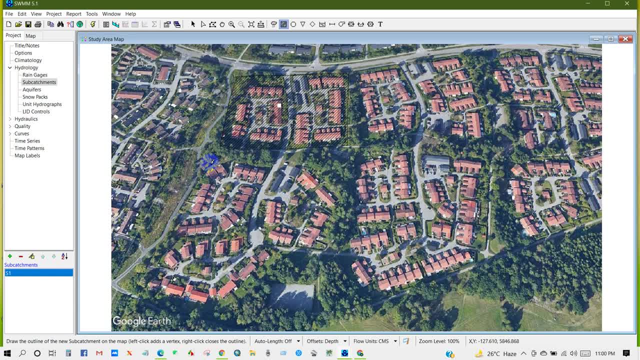 I'll show you how I did it, so enjoy the video. like this: The second subcassment of my study location. When you will stop drawing the right click on your mouse, then it will be stopped automatically and your subcassment will be drawn. 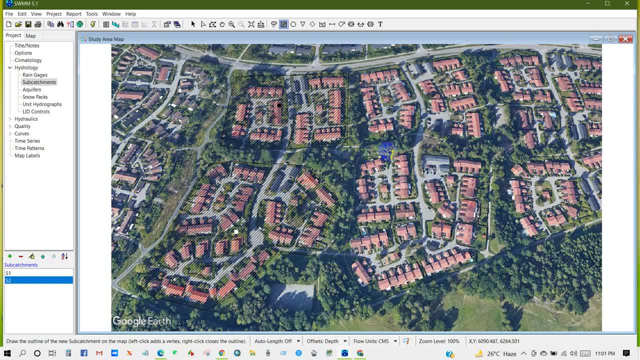 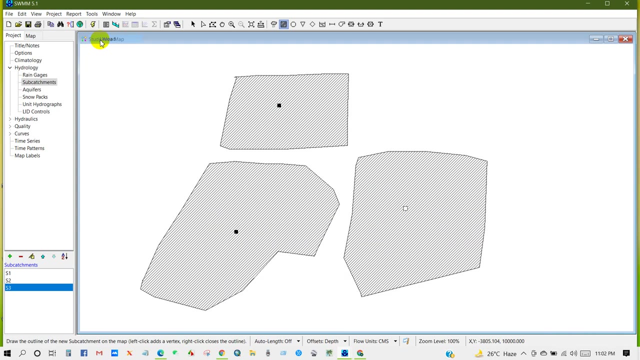 the third number of sub castments of my study area. right click on the mouse after drawing sub castment you can remove the background image for doing that. go to view and then backdrop, then unload. you can delete drawing. right click, then go to options. you can see here map. 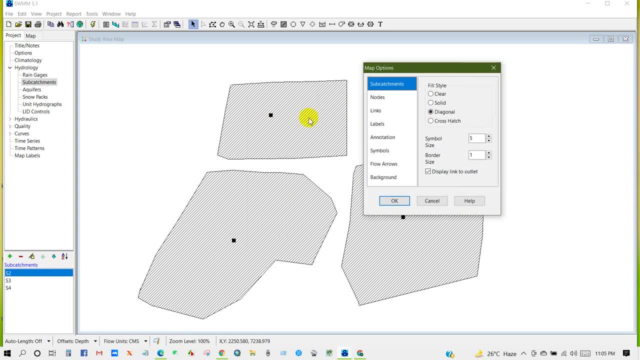 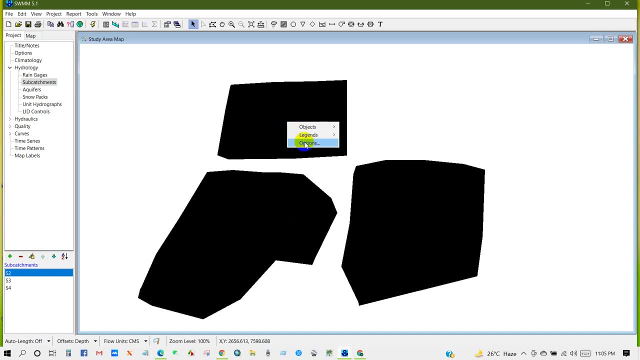 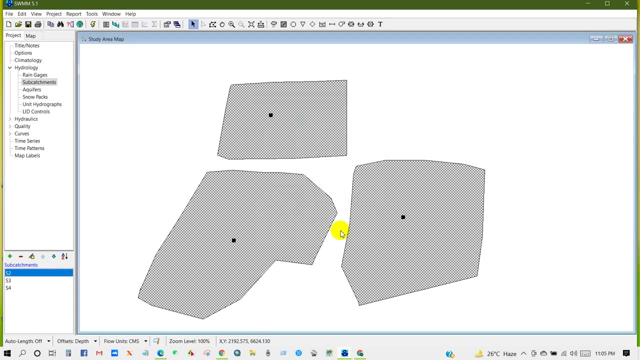 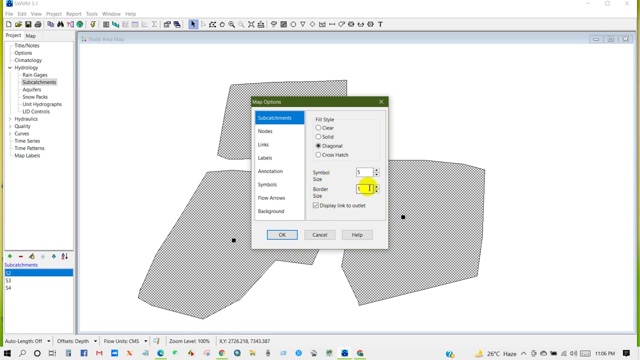 options: sub castment file fill style: you can keep it as solid. then again right click and map options: you can keep it as cross hat. right click on. then options: I'm going to keep it as diagonal. you can increase or decrease the symbol size, border size options: annotation check: sub castment IDs: can increase the font size of sub. 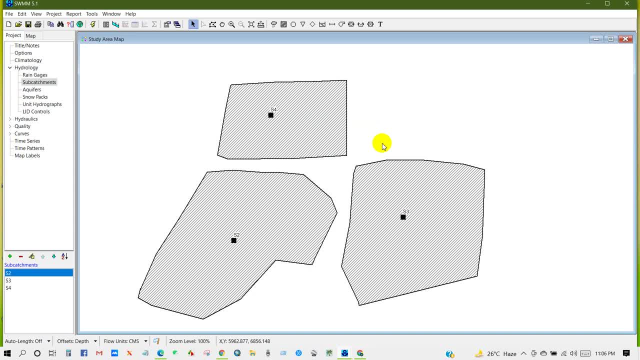 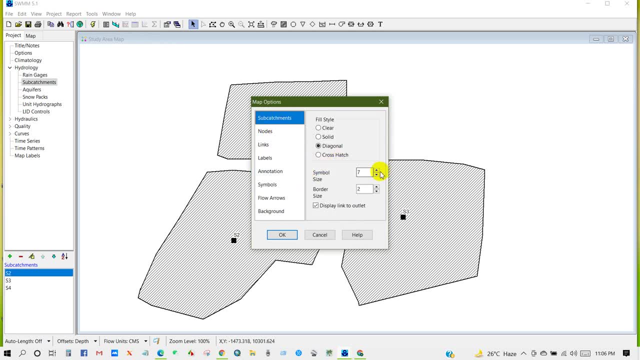 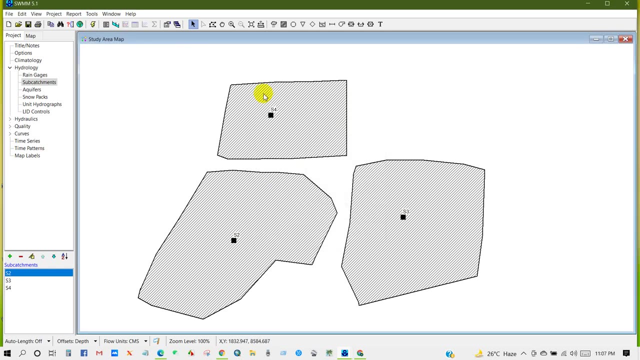 castment IDs. you can go to this option from tools. map display options, from map labels. you can give a specific name for. is sub castment for that map levels. then add object and click in the sub castment. I'm going to give the first sub castment as building one. 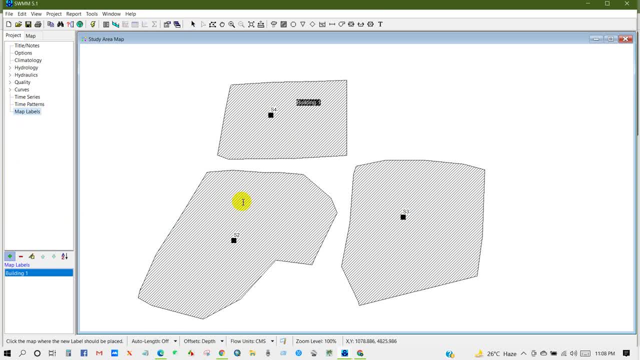 sub castment. for second sub castment I'm going to write building two and for third sub castment I'm going to give it a name for building three. for writing: click enter. I'm drawing three. junction note for three sub castment: updating now finished, so right click on the second sub castment. I'm the open. 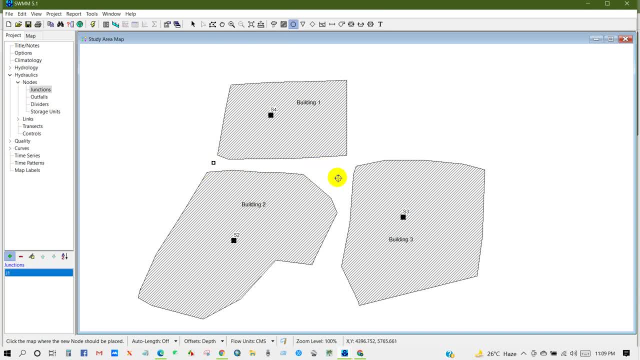 here I need to click on the second sub castment. so here both three gl niego. here I need to click on the seventh sub castment. I'm so I just have to copy this and edit once, click ok and this is at module same and this is the outfall node. 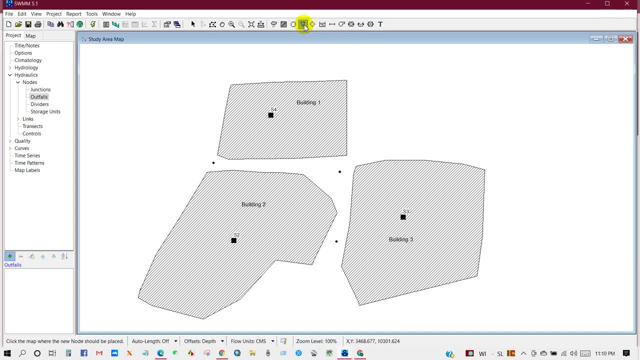 which is in pun겠죠. this is the outfall node. this is the connection node which is in pun Source. so I'm here, I'm going to add value to the connection node. now i i will explain what is node in swmm. a swmm network can include three different types of nodes. 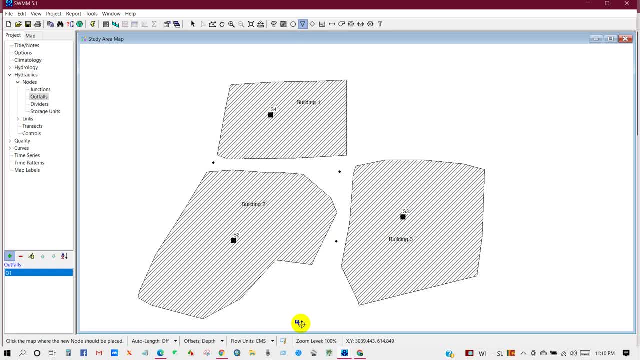 junction, outfall and storage. so what is junction node? junctions are drainage system nodes where links join together. physically they can represent the confluence of natural surface channels, manholes in sewer system or pipe connection fittings. external inflows can enter the system at junctions. and what is outfalls? outfalls are terminal nodes of the drainage system used to. 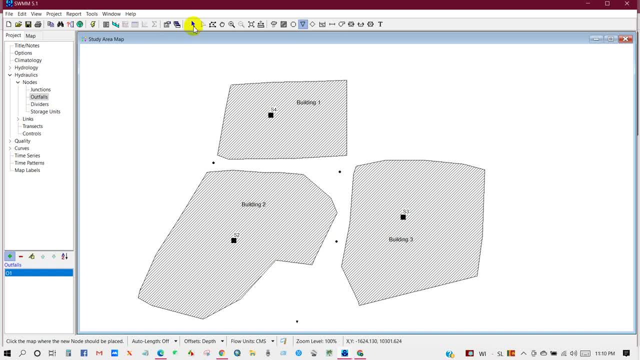 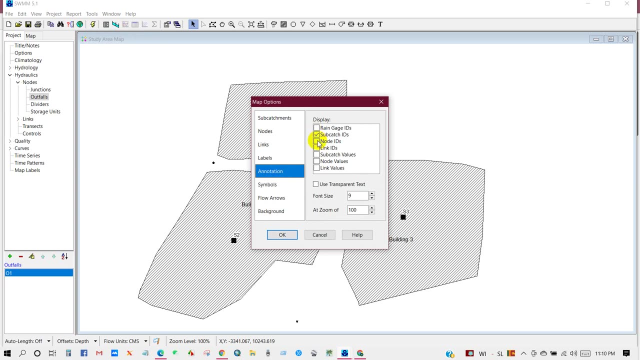 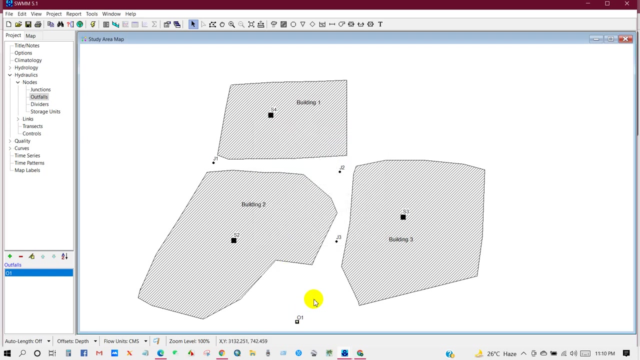 define final downstream boundaries under dynamic wave flow routing. go to tools, then map, display options and annotation. check node ids, rain goes ids and then click ok. now node ids is visible, then add a conduit link. so what is conduits? conduits are pipes for channels that move water from one node to another in the conveyance system. 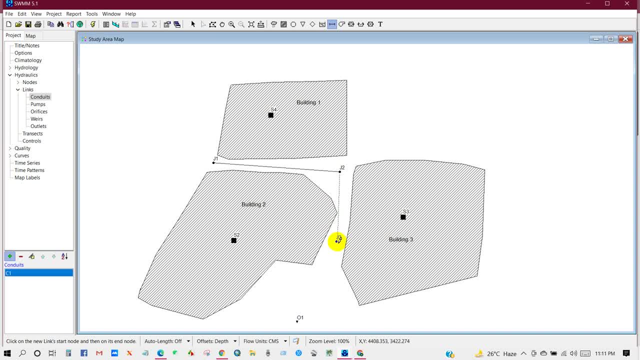 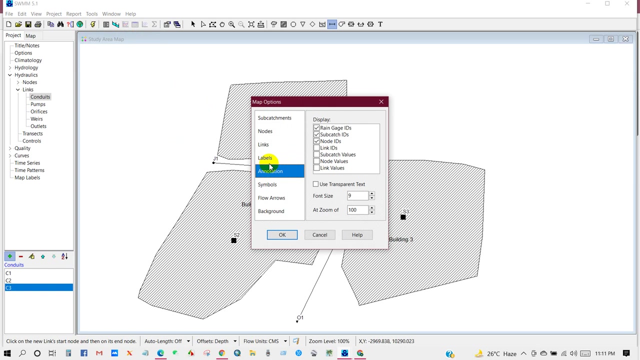 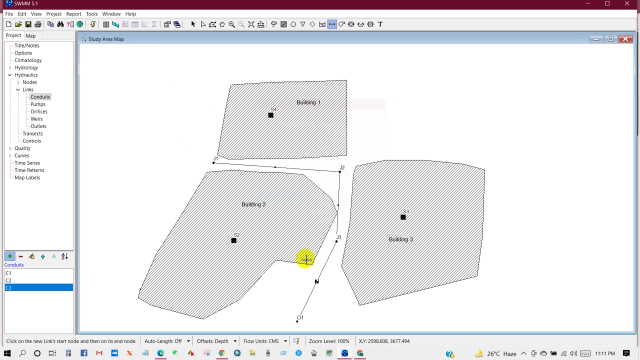 so i am drawing conduits. that means pipeline and connected to all manholes and outfall as well. that means pipeline connected to j1, j2, j3 and finally to outfall, then go to tools and then map, display, option, annotation and theindi my unique personal 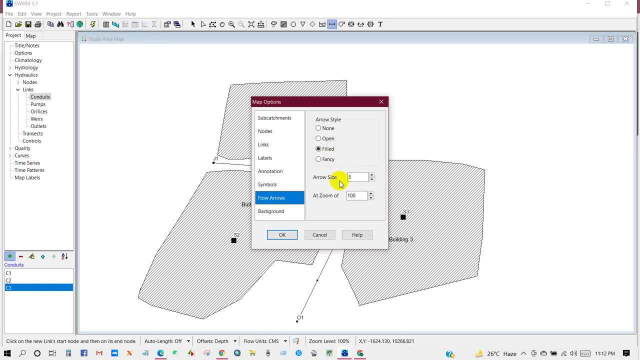 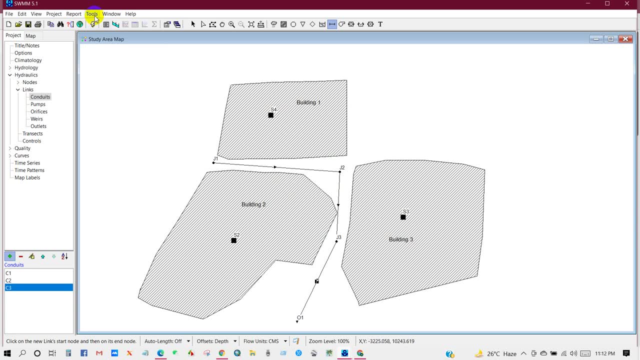 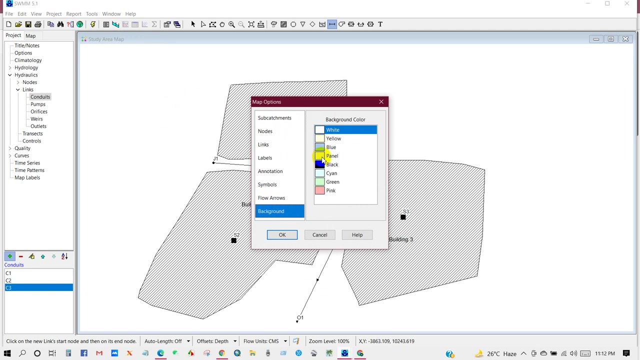 solution: i can ид anis. uh, no, uh, follow arrows. check field. then. okay, you can see here, follow direction. uh, arrow size: you can increase the arrow size, okay, and this pipeline and the link: you can increase the link with single link, the link size. you can change the background color. 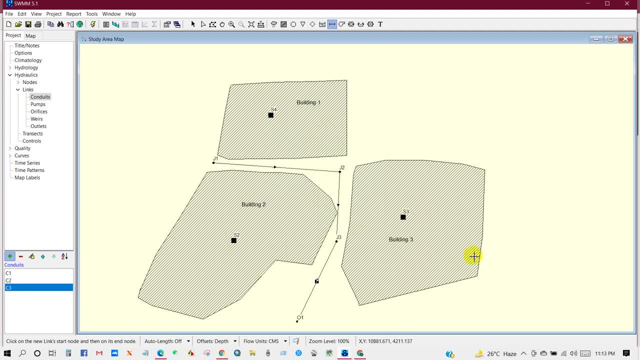 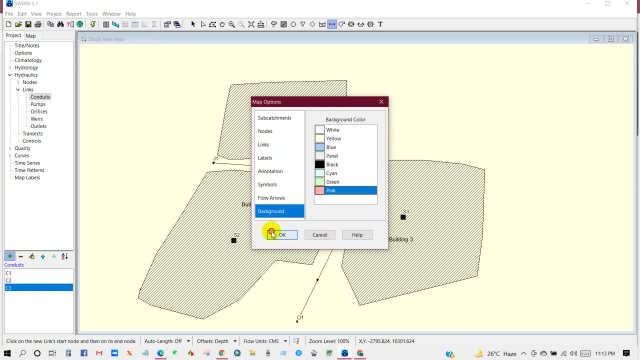 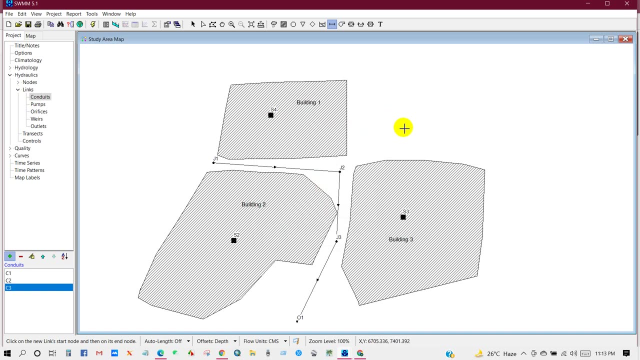 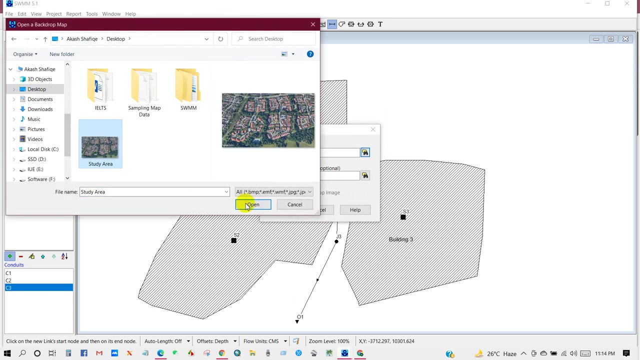 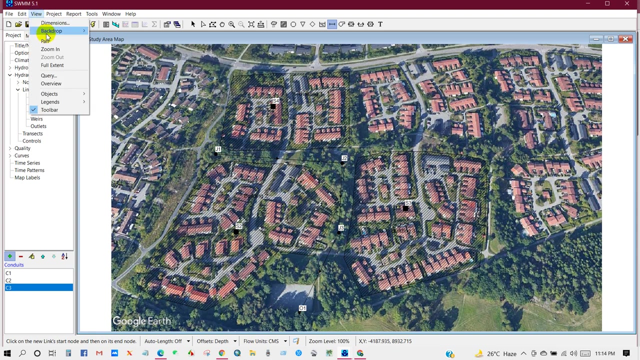 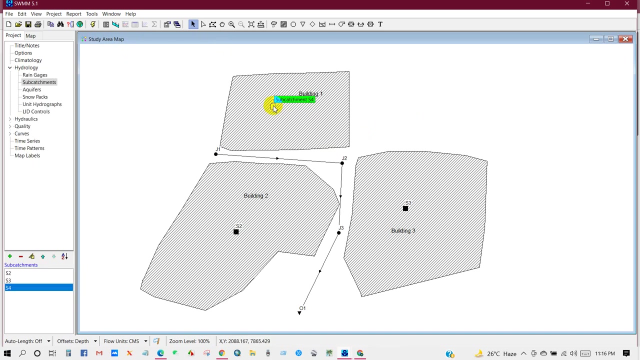 from map display option: background color. I'm keeping it as white. nodes: you can increase the nodes. node size: node size has been increased. you can load the raster file again now. I will link the subcastment to junction. so here changing the name, subcastment is one. 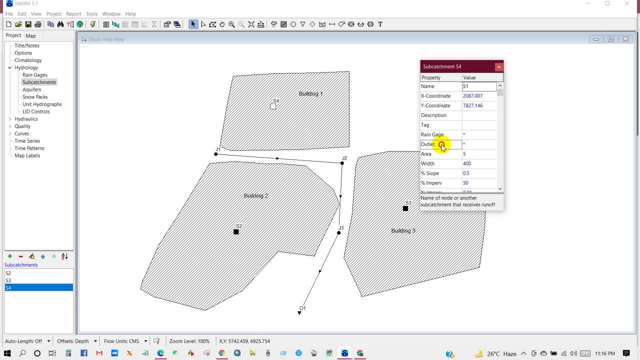 first subcastment in outlet for first sub castment outlet will be j1, junction one. you can change uh, you can uh. you can change uh, you can uh. define the area with slope and so many things here you will find it depends on your study area and your design. 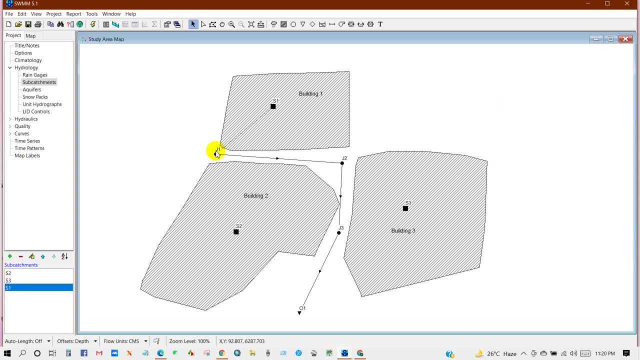 then uh, second, uh castment, subcastment. so second surface name is two. it can uh give here several information. so for second subcastment the outlet will be junction two and then area 32 j three. so this is the different submit subcanvas. and then uh. for third sub assessment the junction node will be uh j three. 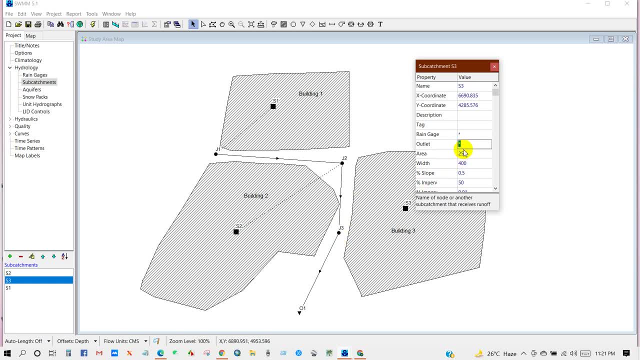 define area, then outlet will be j3 junction node, i mean the manhole, so subcastment, and note here invert elevation. for first junction I'm giving invert elevation 7.2 meter. you can also put here maximum depth, initial depth and others information as well. for junction 2 I'm giving invert elevation 6.7. 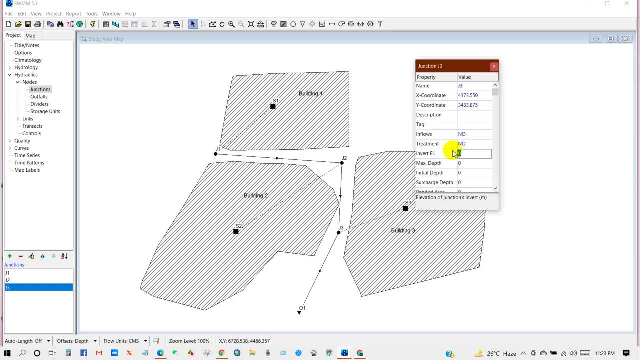 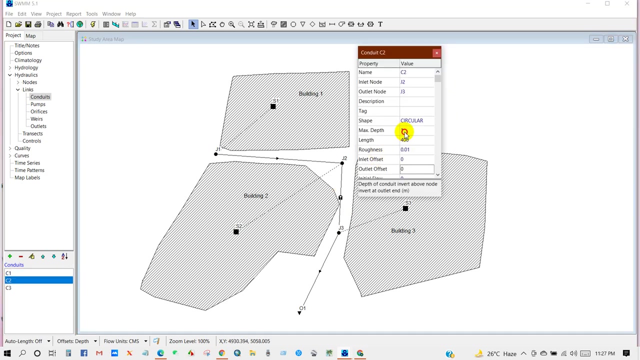 junction 3. double click on this and then invert elevation 6.2 for junction 3 note. then for outlet I'm putting same value of bothś you can also put here position here. then波leg me evenلا. invert elevation, thenž invert elevation. 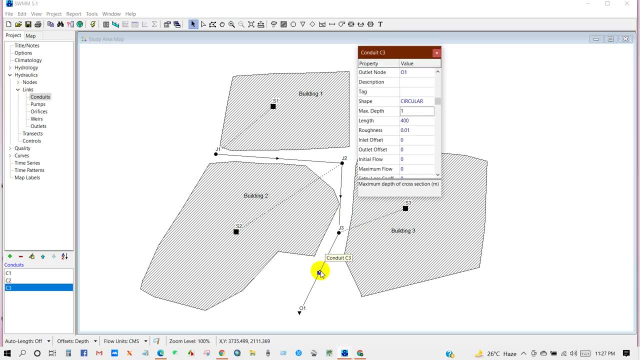 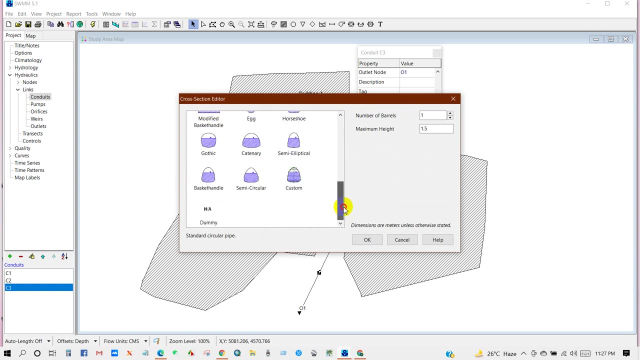 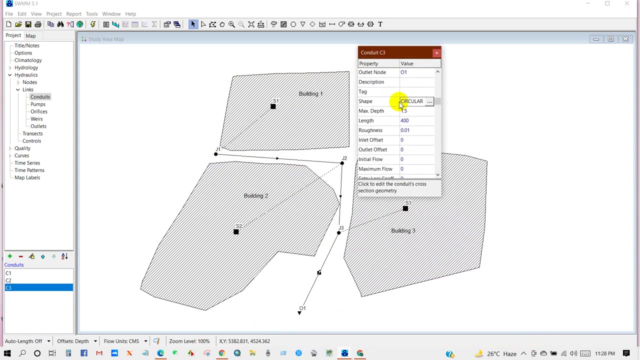 mean depth for pipeline. I'm giving 1.5 for earth conduits. conduit I mean pipeline shape. you can see here several shape of pipeline: rectangular, triangular, parabolic, force main circular shape close to rectangular. I'm selecting circular shape for my conduit. now I will add a. 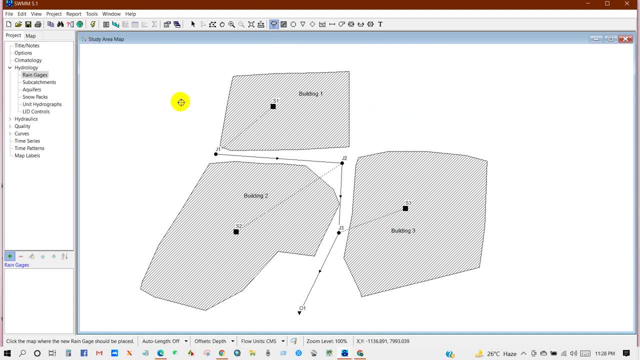 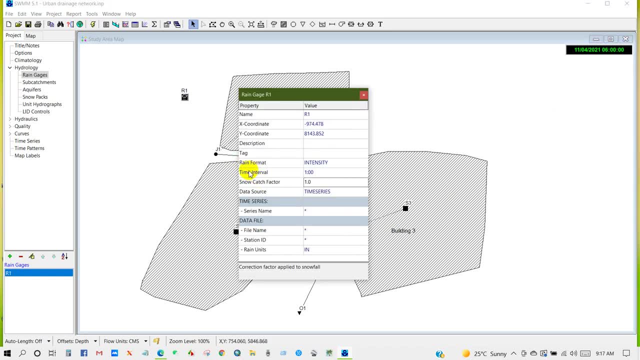 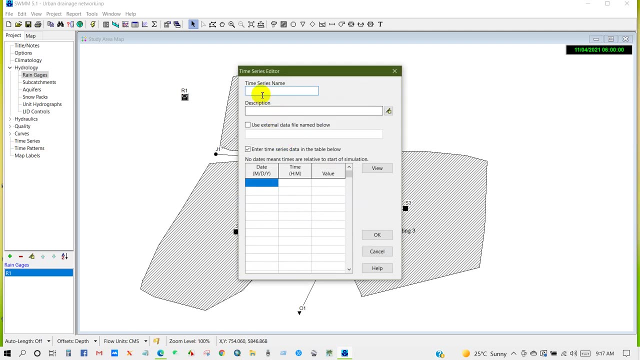 random rain gauze. rain gauze is supply precipitation data for on or more sub-cast materials in a study region. the rainfall data can be either a user defined time series or come from an external file time series. add rain data here. time series name: five year written period. then add time. 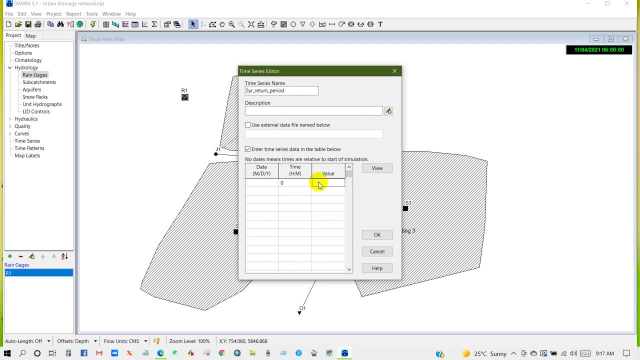 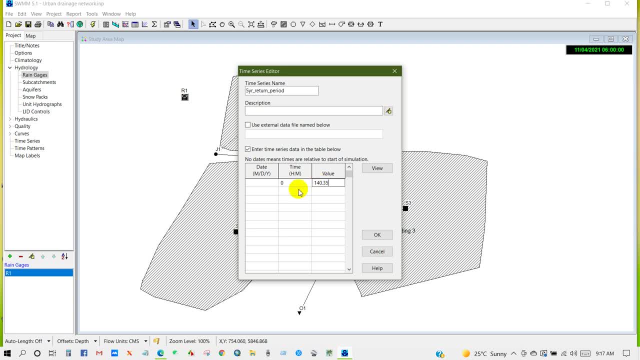 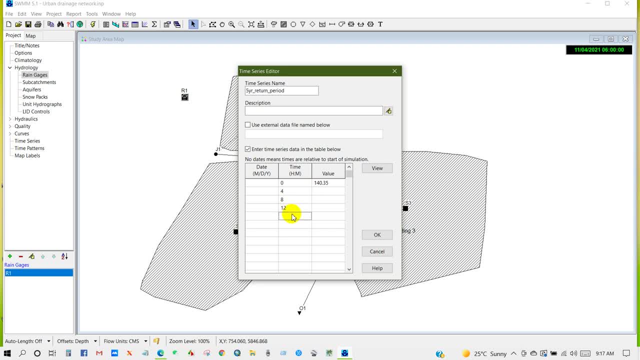 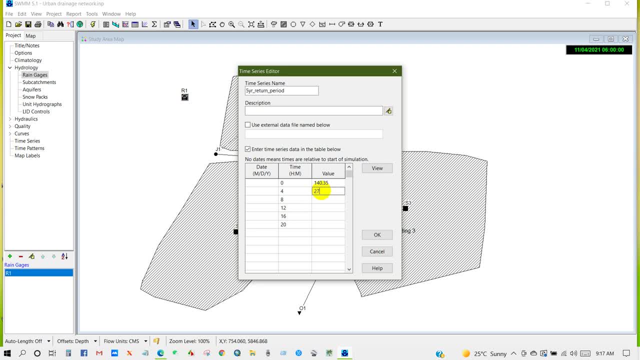 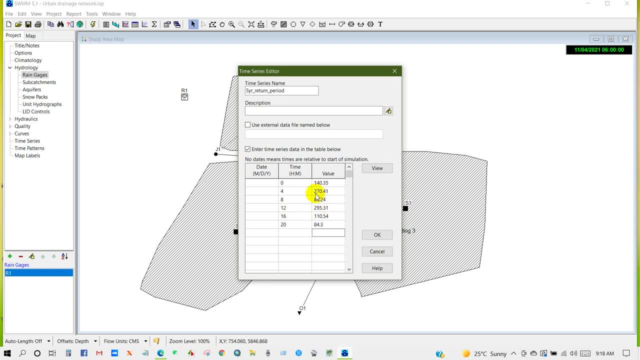 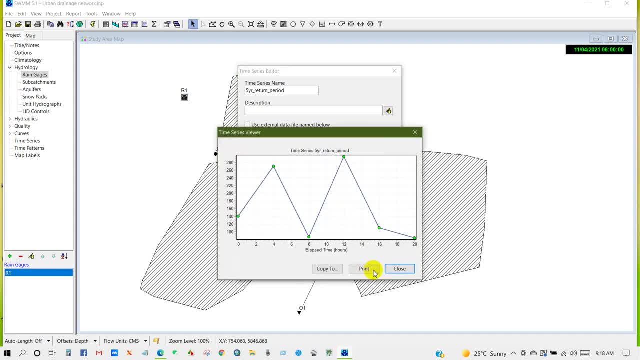 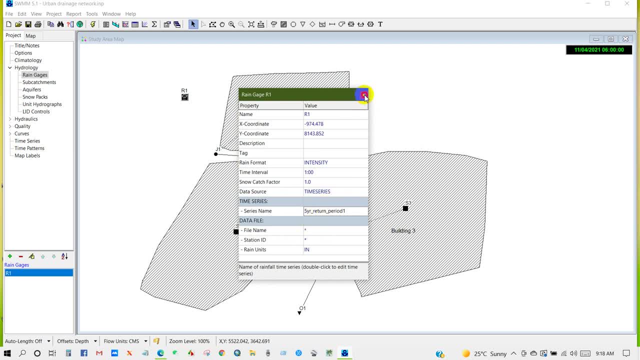 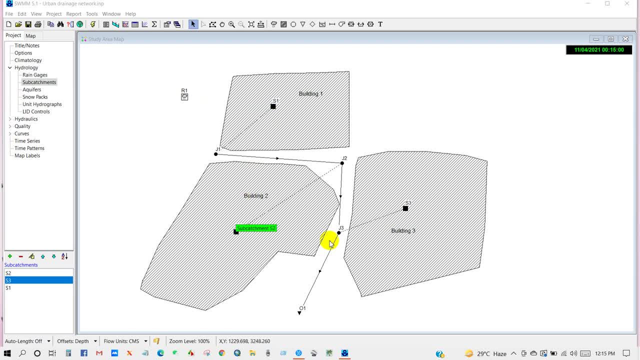 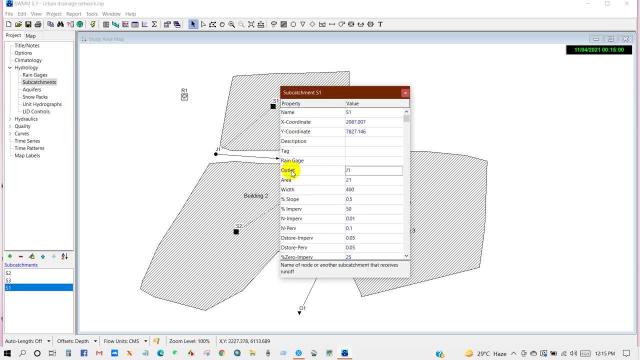 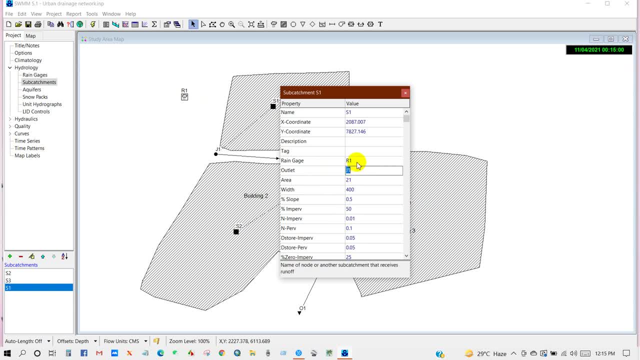 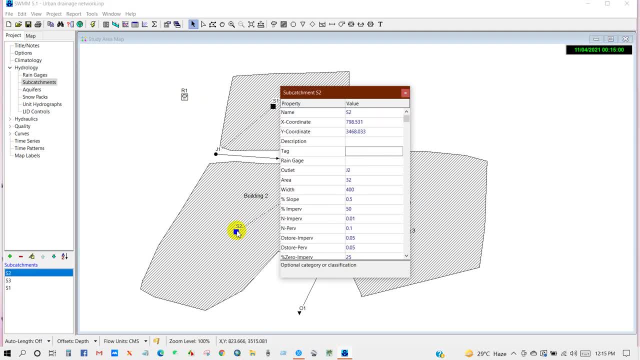 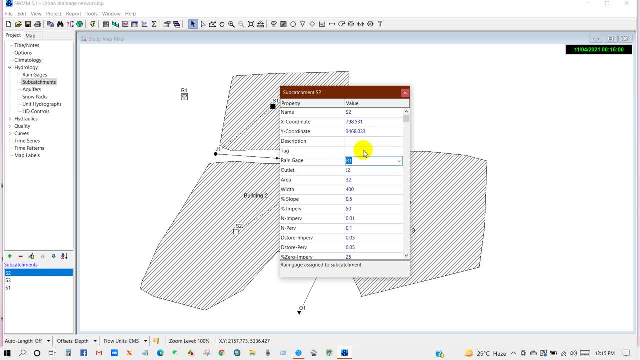 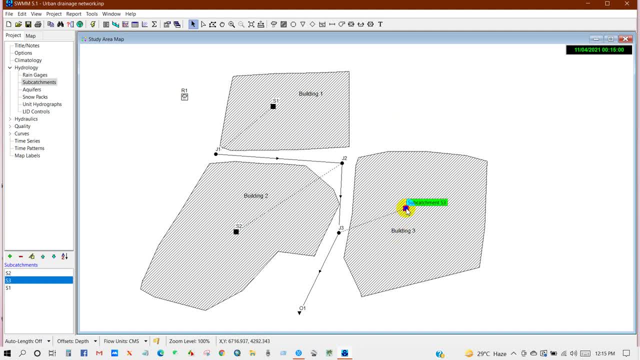 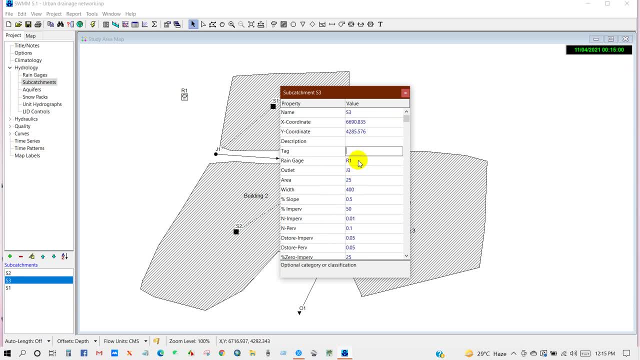 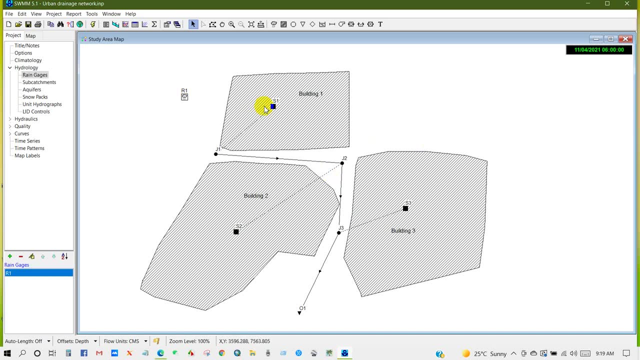 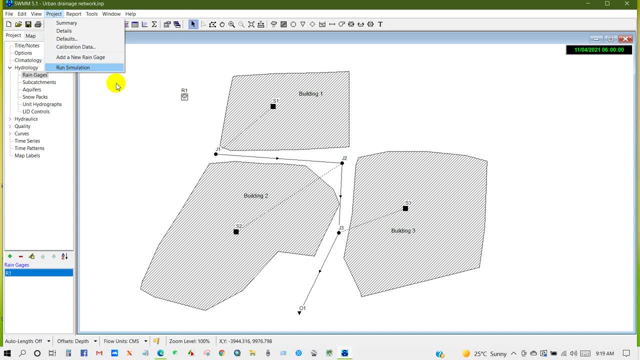 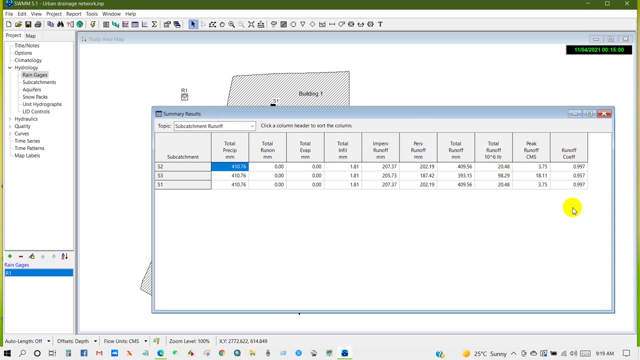 run simulation from this option or from this option. so click run simulation and run simulation successful with some errors. click here summary results. you can see here summary results: subcastments, runoff, runoff coefficient. then node depth: maximum azl meters. average depth meters. so many information here. you can uh get information. 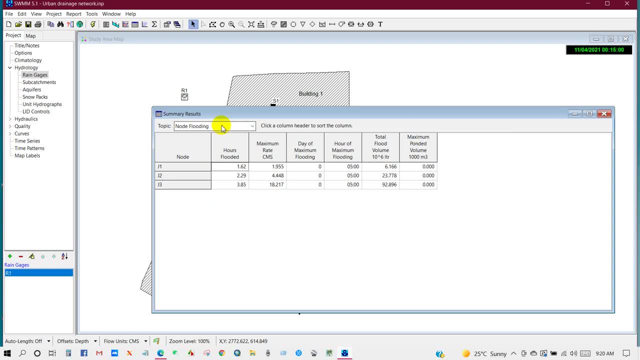 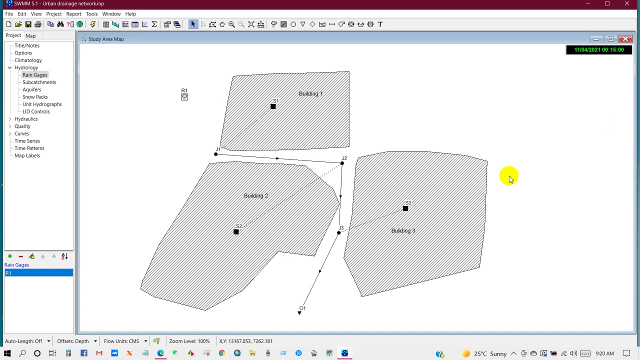 and essentially information from here for your research purpose. node flooding, outfall, loading, link flow, maximum flow, minimum flow conduit search charts. distributionDoesn't affect water cellgrain. create a profile plot, then initial node, then outlet end node and find path to 3 conduits. then click ok. then you can see water elevation profile. 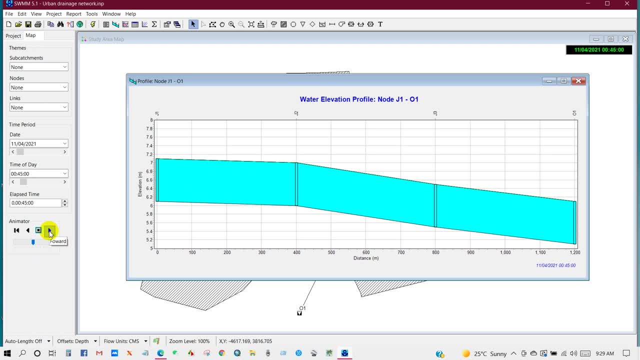 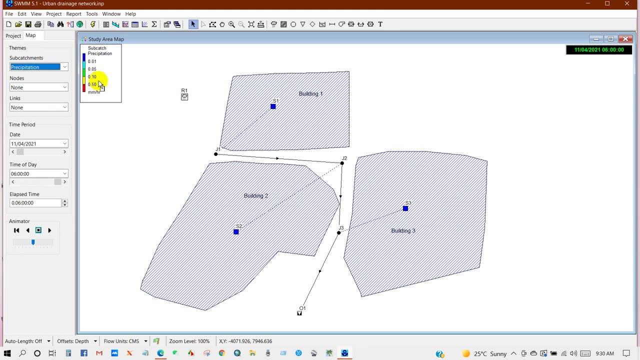 then click map. if I click on run animation button, you can see how water elevation works based on time code page on time. now select precipitation for sub-casements, then depth for nodes and flow for links. once we clicked on the animation simulation, we can see how the 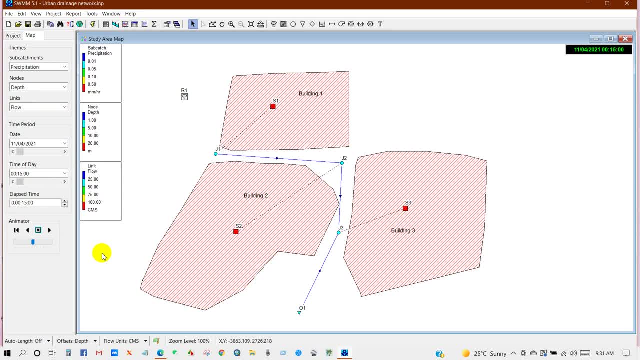 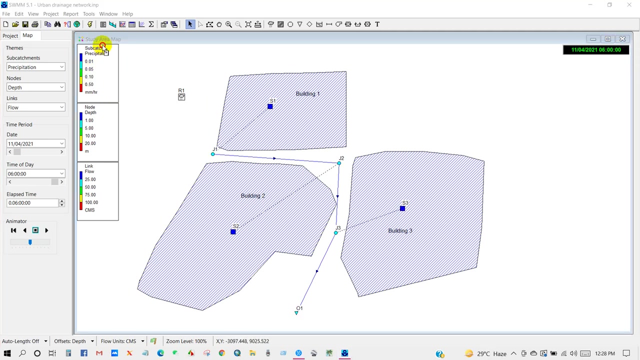 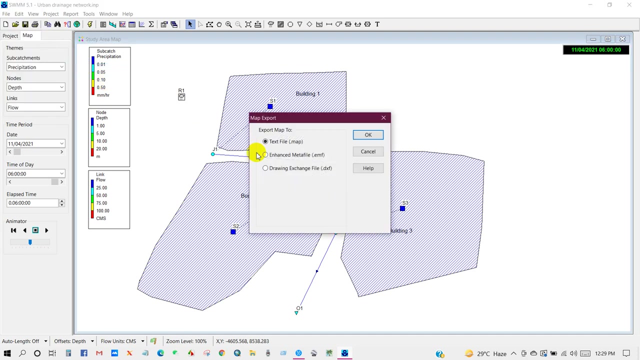 pipe. pipes change in color as the velocity of the water changes. right click you can change color. дисam. you will find here several options: framed or unframed. then you can a print the file or you can save the file from here. you can export the file as map. then you can export map to text file enhanced. 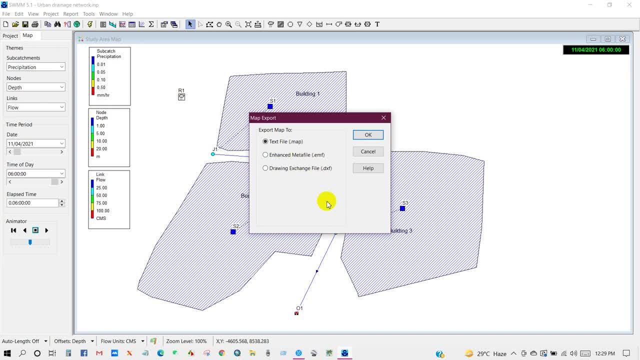 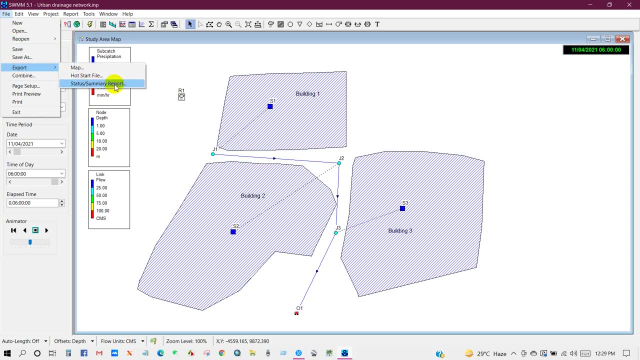 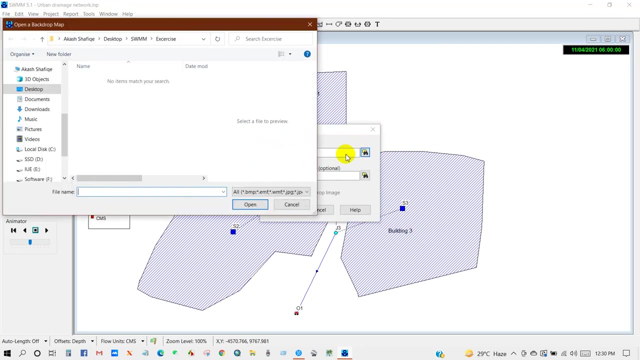 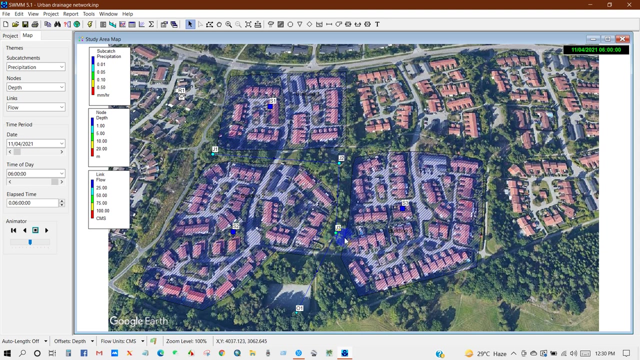 meta file or drawing exchange file. you can see I can save summary results from here. screen preview. you can bring this file from here. again you can load the raster file. I hope you guys got a clear idea about HWC HWMM model. I tried to show you how you can design an urban drainage system- the 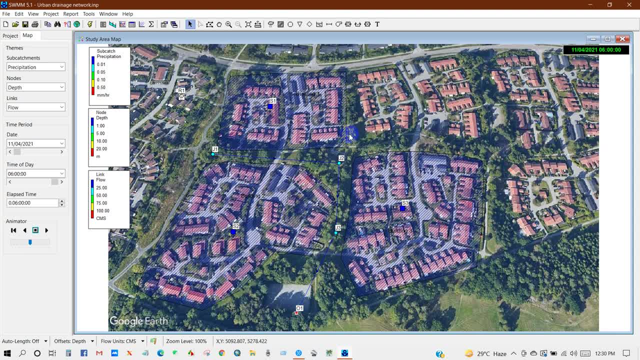 data I have used in this model is for just an example. I hope you learned how to draw manholes, pipes, subcastment and set rain gauze, adding data for all objects, and how to run the model and get data for your research or project purposes. in the help menu of HWMM you will find manuals and many useful. 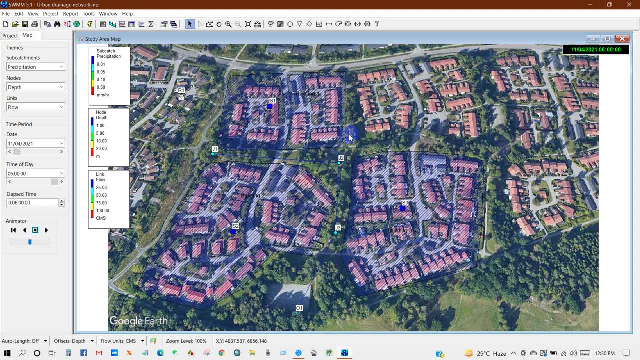 information. anyway. in the next video I will show you how you can design urban drainage system for more than six subcastment. till then, stay safe and thank you.